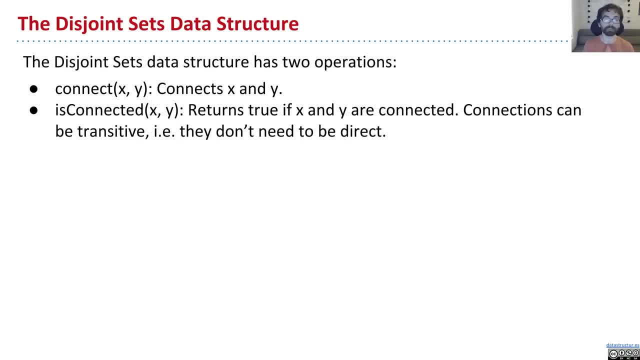 So let's jump into what the disjoint sets data structure is. So it has two operations. The first is connect, which connects two items, And the second is isConnected, And it returns if two items are connected. Now connections can either be direct: 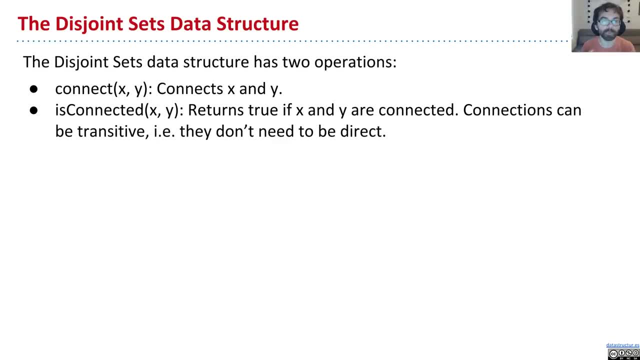 or they could be indirect. that is the result of a bunch of transitive connection operations. So, for example, let's suppose we connect China and Vietnam in our data structure And then we connect China and Mongolia And then we ask: is Vietnam and Mongolia connected? 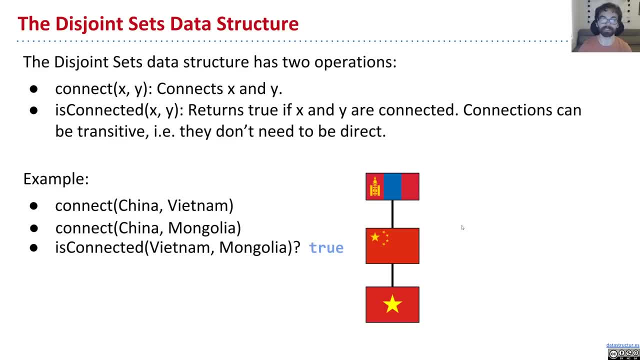 Yes. Well, the answer is they are indeed, because we have a transitive set of connections. If we then say, let's connect the USA and Canada and then check whether the US is connected to Mongolia, the answer here is false. 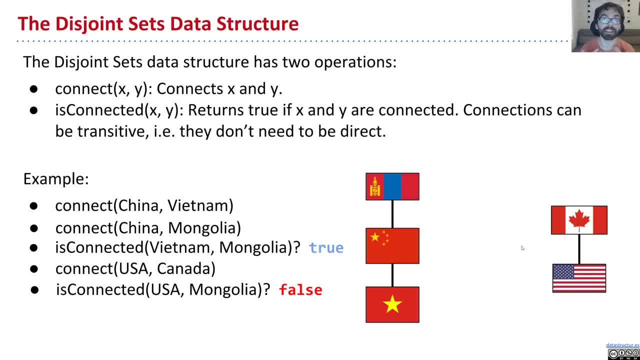 And you and I can see that visually, But we're going to be building a data structure in a computer that can solve that same problem. Now the answers can change. So, for example, let's suppose we connect up China and the United States. 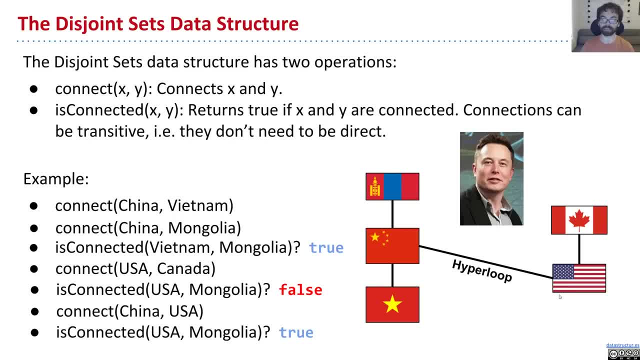 In that case, if we now ask if the United States and Mongolia are connected, we would say true, That's it. That's all we're going to do today is build this data structure with these two very simple operations. Now you might say: why would I ever want this thing? 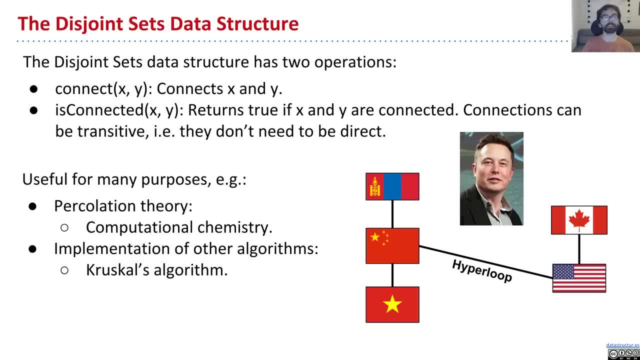 And it turns out that this is useful for many of us, For many purposes. One of them is in the natural sciences, somewhat surprisingly So, there's an area known as percolation theory. Actually, this also comes up in pure mathematics and applied mathematics. 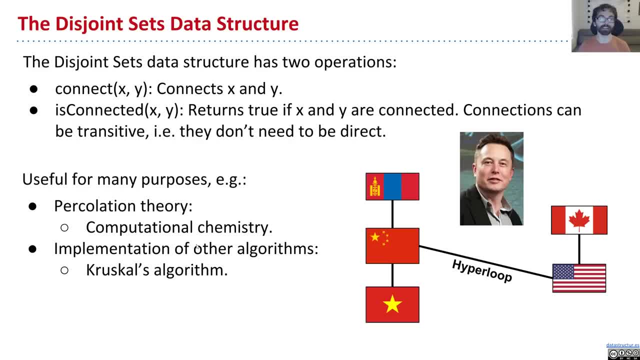 And one of the most interesting examples that we'll actually see in the homework in this class is a computational chemistry problem that this data structure will enable us to solve. It's also useful as a basic building block for other algorithms, For example, an algorithm we'll talk about later in class. 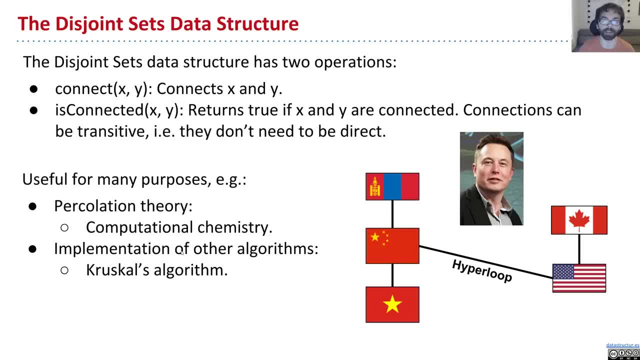 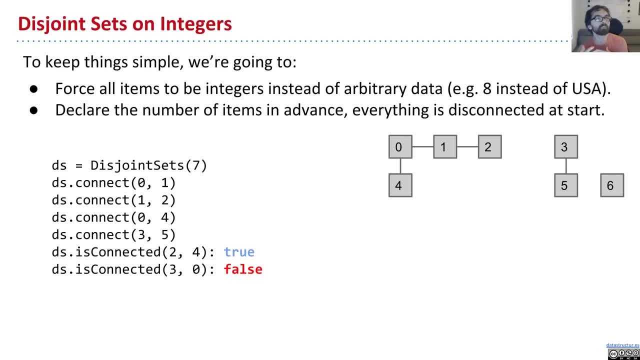 known as Criscoll's algorithm. So it turns out to be a generally useful thing. So I'm going to simplify the problem just a little bit in order to make it just simpler to think about. There's no loss of generality here. 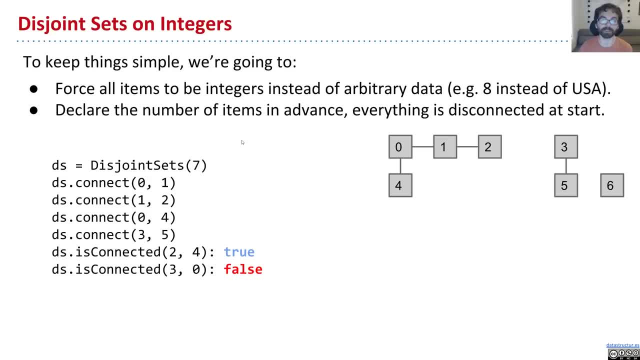 But what we're going to do is we're going to force all of our items to be integers instead of arbitrary data. So we can't just connect USA, We're instead going to say connect up 8.. So all my items are going to be all integers. 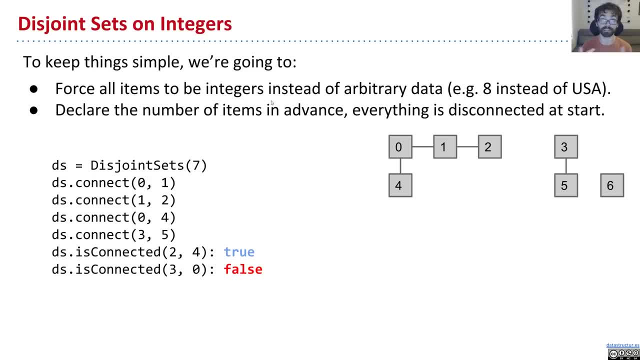 And then, secondly, we're going to say that everything must be declared as existing in advance. So I'm going to, for example, say I want a disjoint sets object of size 7. And everything will be disconnected at start And then, after I connect up, 0 and 1,, 1 and 2,, 0 and 4,, 3 and 5,. 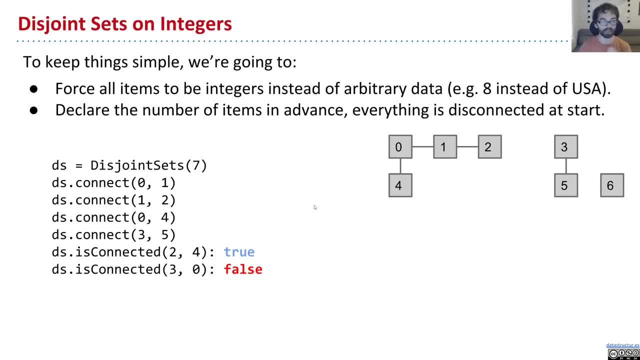 we end up with this topology Now, just as we saw in the USA, China, Mongolia, Vietnam and Canada example, we can now call, say isConnected And say: are 2 and 4 connected? Yes, Are 3 and 0 connected? 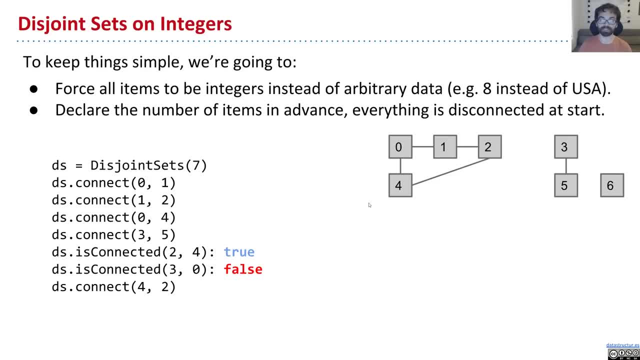 Nope, And just as before, we can connect things up. Let's connect 4 and 2.. Let's connect 4 and 6.. Let's connect 3 and 6.. Hooray, Now if we go through and say: are 3 and 0 connected? 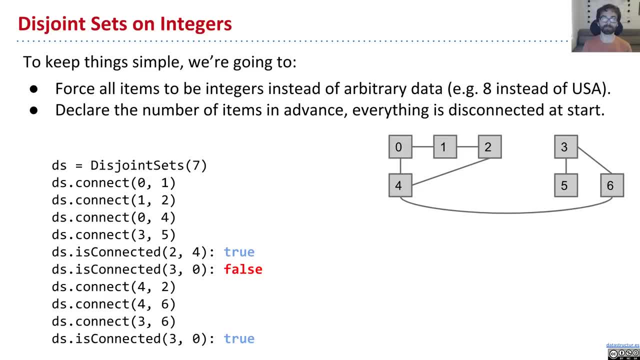 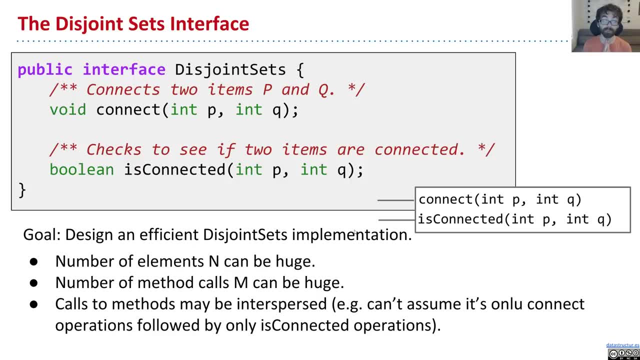 The answer is now true. So how do we make this thing? What's it going to look like? Well, I do want to address the issue of we're going to ultimately be writing Java code, And so the interface we might have in Java. 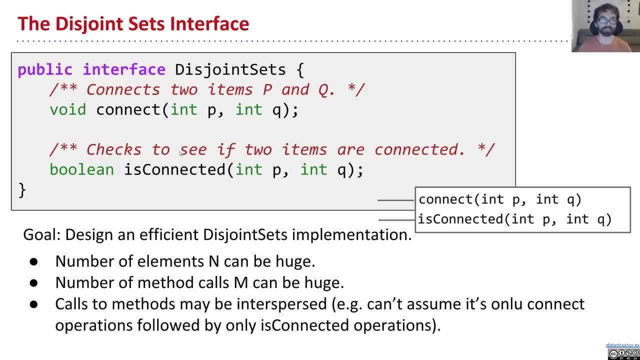 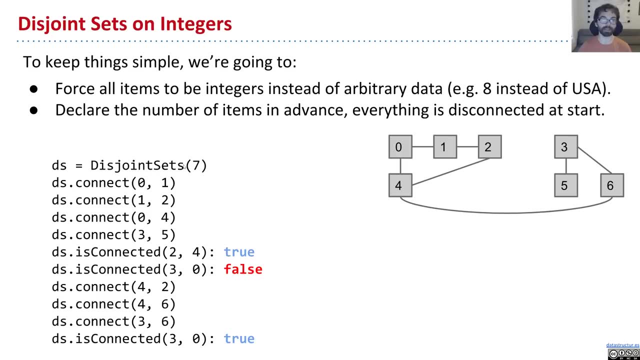 would be something called disjoint sets. That has a connect and it is connected operation. And now our goal is to actually build the specific implementation of this disjoint sets interface. Now we have to keep in mind a few things. One: the number of elements in our disjoint sets. object: 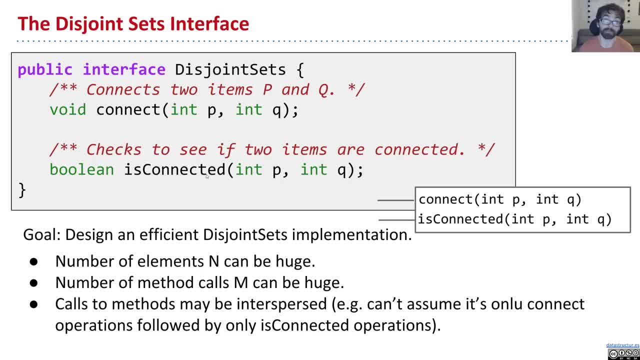 right here could be potentially huge, let's say millions or maybe even hundreds of millions, And the number of method calls can also be huge. So it won't be good enough just to do some brute force thing. We're going to have to be a little more clever. 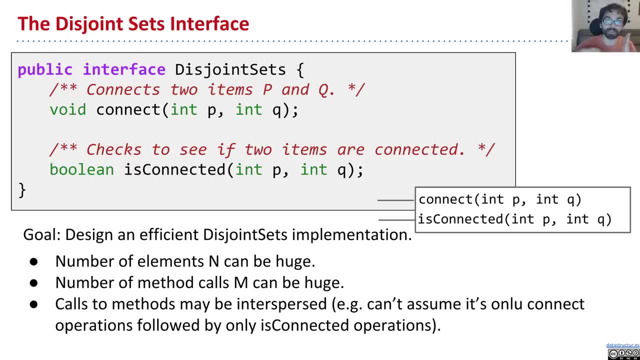 And we also need to keep in mind that the calls to the methods can be interspersed, So it's not like someone's going to do all the connections first and all the is-connecteds first, And that would actually result in an easier data structure. 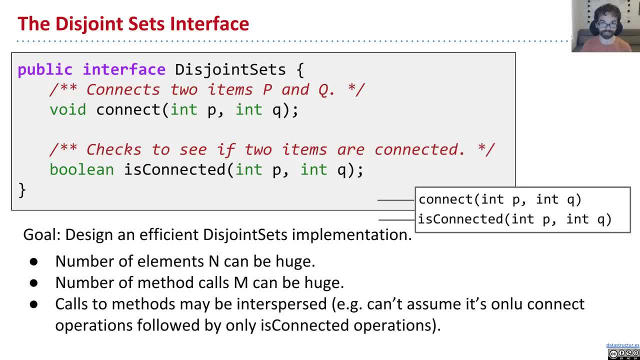 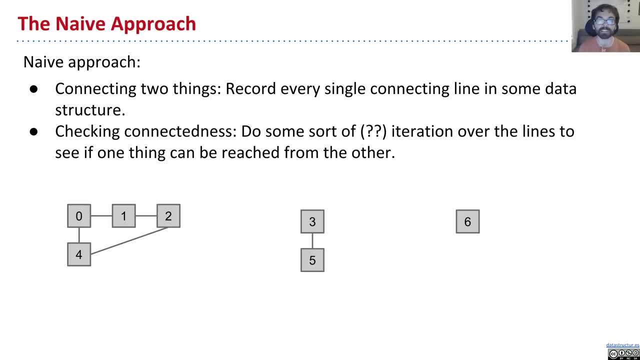 But because we have to deal with dynamic connectivity, that is, it can change over time. it'll change the way we approach the problem, as we'll see. So let's start by considering just a naive approach to finish our setup And, in this approach, what we would. 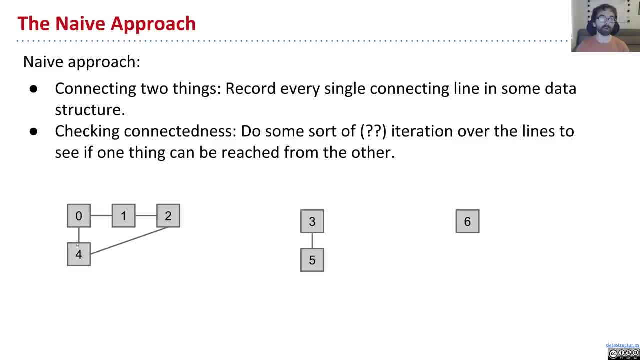 do if we wanted to connect two things is we would record in some kind of data structure all the lines connecting every individual connection And then, when we called is-connected, we would do some kind of iteration over the lines, Like, let's say, we did is-connected 0, 5.. 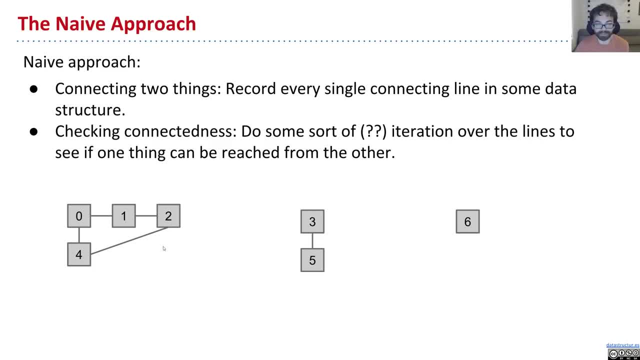 We would do some kind of maybe recursive thing where I look at the neighbors and then do something. But I'm actually going to stop us right there. This is too much, And I'm going to make a really important observation that's going to make our lives much better. 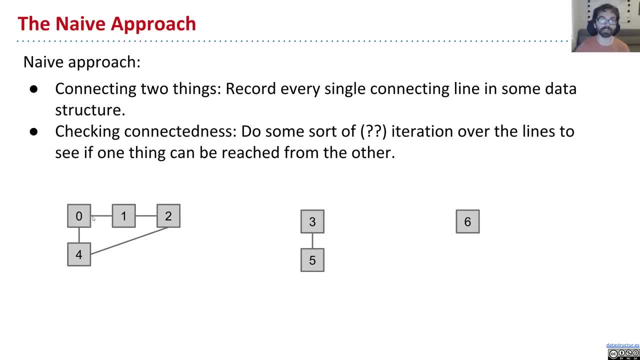 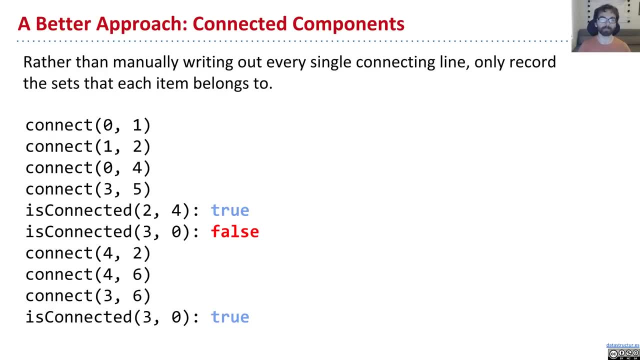 Specifically. we do not need to actually do this, We do not need to actually keep track of each individual line, But instead we can keep track of only the sets that each line belongs to, Or sorry, only the sets that each item belongs to. 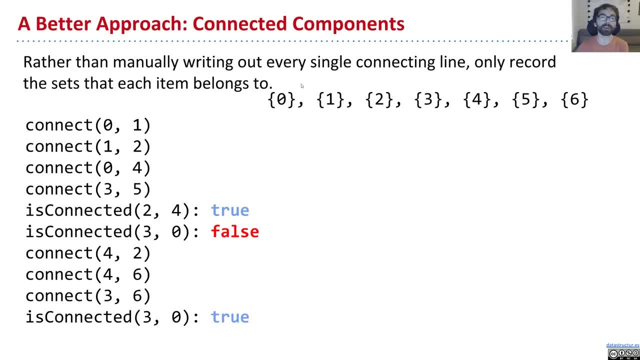 So if I say connect 0, 1,, at that point we go from everything belonging to its own individual set to now 0 and 1 being part of the same set. When we connect 1 and 2, we bring 2 into that set. 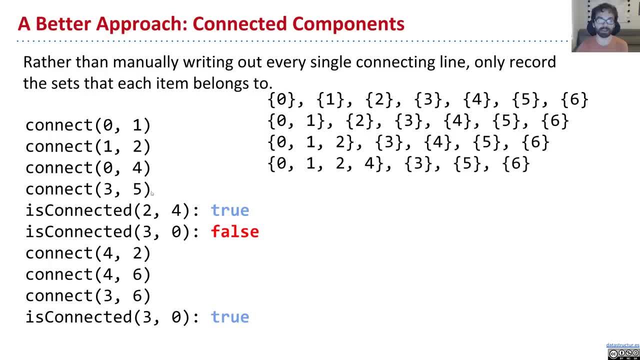 When we connect 4, we bring 4 into the set. When we connect 3 and 5, these two sets are merged. At this point the is-connected operation just says: are they in the same set? And it's a little different than what you might have tried to do. 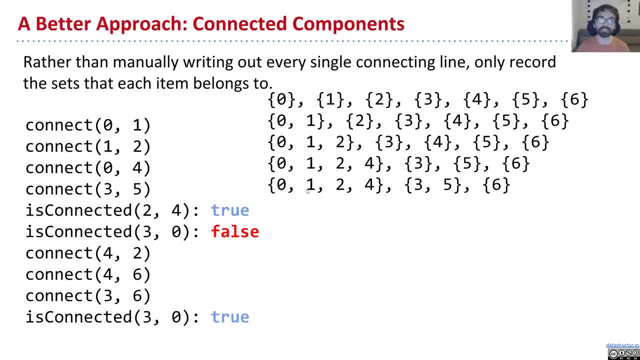 naively where you had all these lines you had to think about. This is simpler. So next up, if we connect 4 and 2, you can try and think about how the state of the universe changes. Turns out it does not. 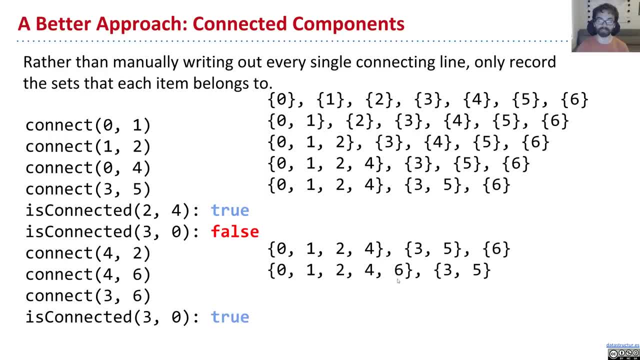 They're already connected. If we connect 4 and 6, 6 gets brought into the set. And then we connect 4 and 6, 6 gets brought into the set. And when we finally connect 3 and 6,. 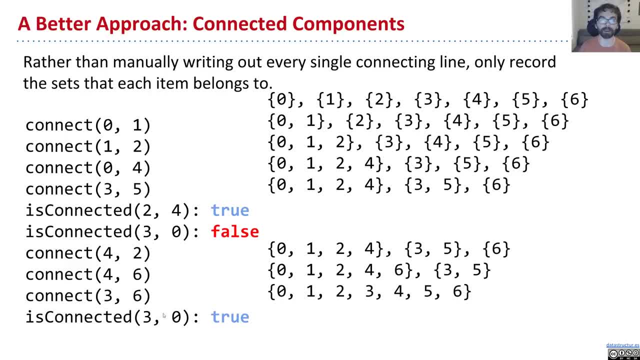 everyone's part of one big happy family and all is-connected operations will return true. So the big idea here was: if we only keep track of the sets that you belong to, then hey, the problem is a little easier. We don't have to write down the line.